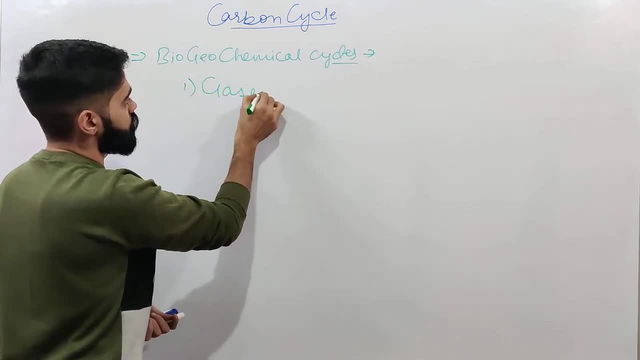 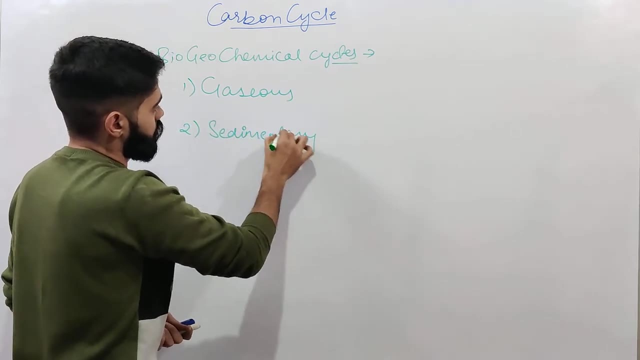 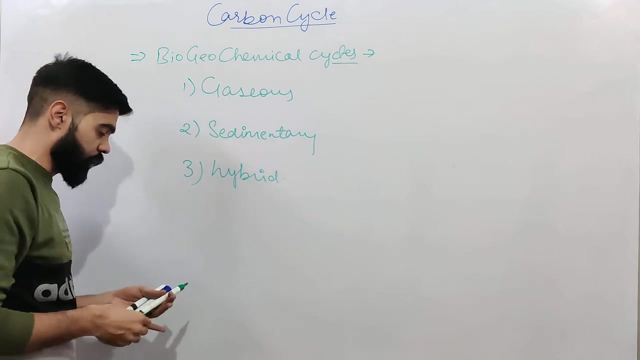 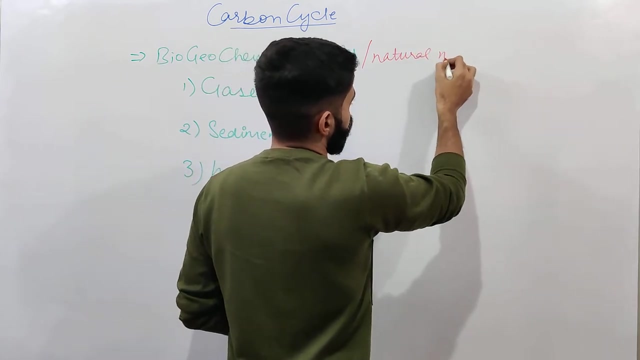 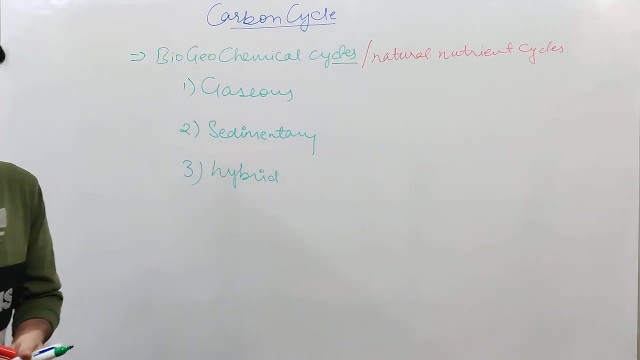 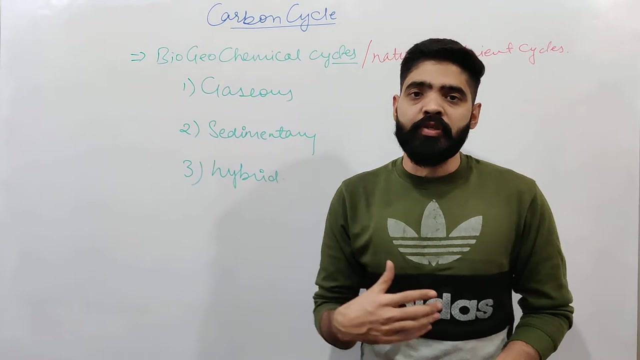 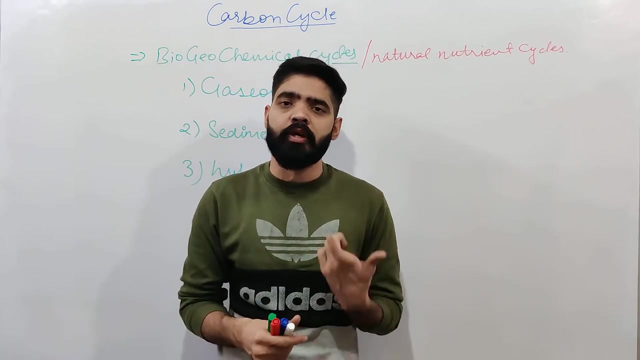 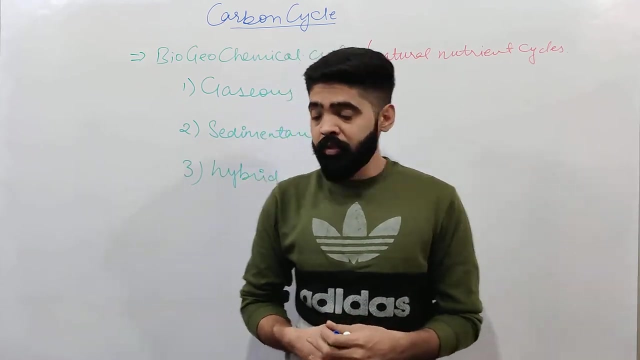 One we have is gaseous. Second we have is sedimentary. Third we have are hybrid. Hybrid cycles are also present in these conditions, in natural conditions. These biogeochemicals are also known as natural nutrient cycles. Clear with this, Natural nutrient cycles. Now see if we talk about the questions from the ecosystem. the complete ecology contains 14 marks and the part of NEET contains 10 or 12 questions from the ecology. That is equivalent to either 40 marks or 48 marks Out of total 360. Clear with this. 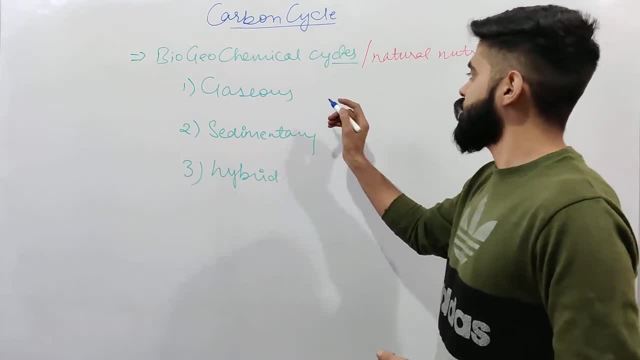 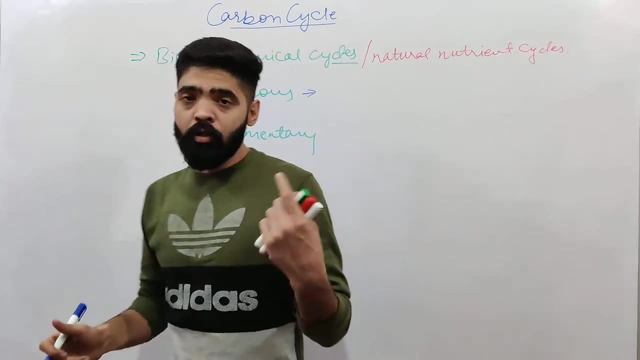 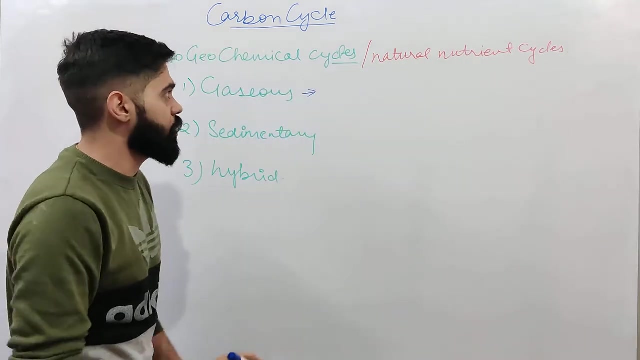 So whenever we talk about the gaseous condition- and we have seen these questions many times- One year is left and one year is repeated. So I am going to also tell you which type of questions are included in NEET from these complete biogeochemical cycles or nutrient cycles. Talking about gaseous one, 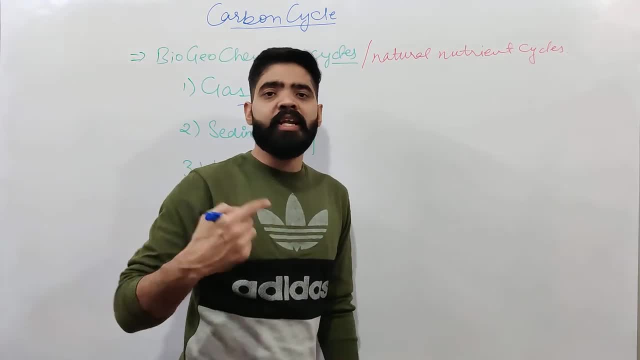 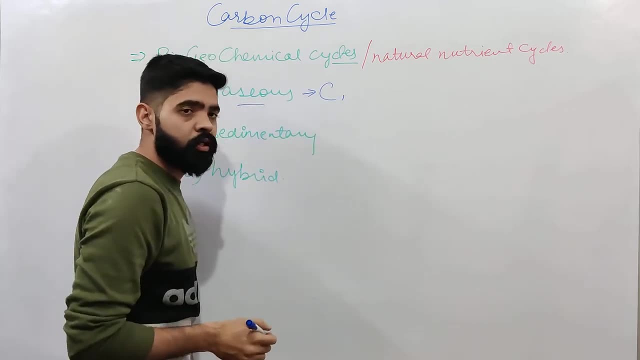 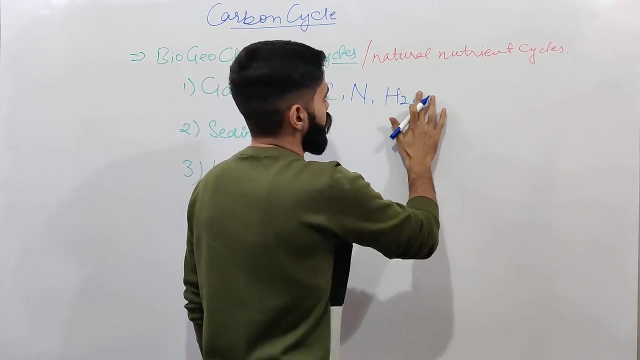 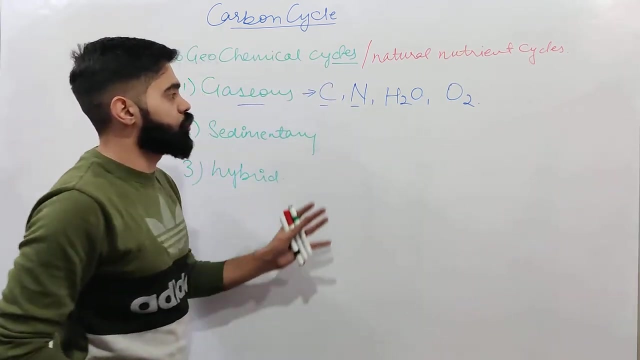 Anything which is present in the environment and can be regulated from the environment are known as gaseous cycles. One we have is carbon cycle. Second in this regard is nitrogen cycle. Third is hydrogen, ie, H2O, And fourth is oxygen. Now see, Whenever we talk about the carbon and nitrogen, and these two are very much important for a plant. 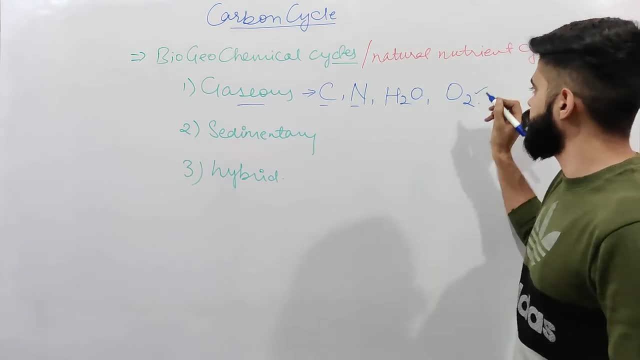 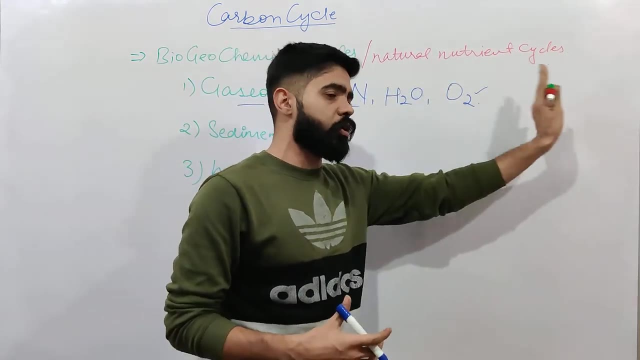 And water and oxygen are also responsible for it. primarily, oxygen is a waste material and also produced during photosynthesis, So we can keep the oxygen cycle aside for plants. only once, Talking about water, Was the water in the same or not present condition with both? 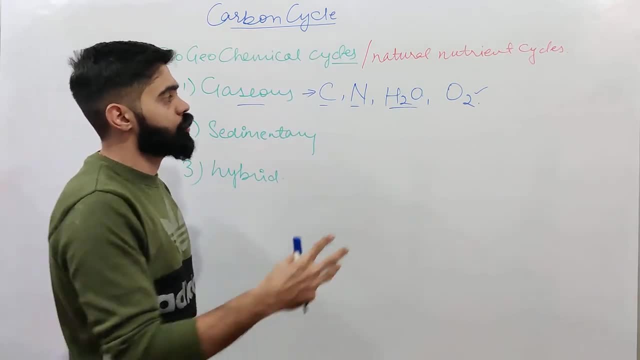 Is there water in the same or not present Least? we can put it in the wrong advantage, We can put it in the wrong position. So the After-sale cycle is caught in the also match with the water component. in both conditions And near the other condition, the cold is less. 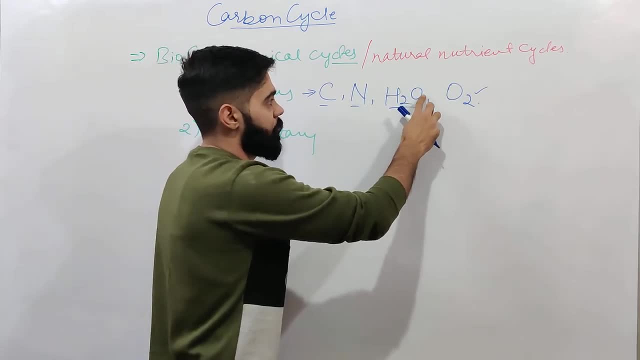 If you observe that we have a fire below the blood, is there with put under the water or not? For that we stem the hydrogen cycle, whether it is present in the water or not present, And ash perdosp Punkt 2.. but we don't use water cycle in this way because water is a non-nutrient material. actually, all of these four are non-nutrients, because the reason behind calling them non-nutrient elements is that they do not uptake from the soil. and whatever is not uptake from the soil, we call them non-minerals or non-nutrient minerals. these are the basics. 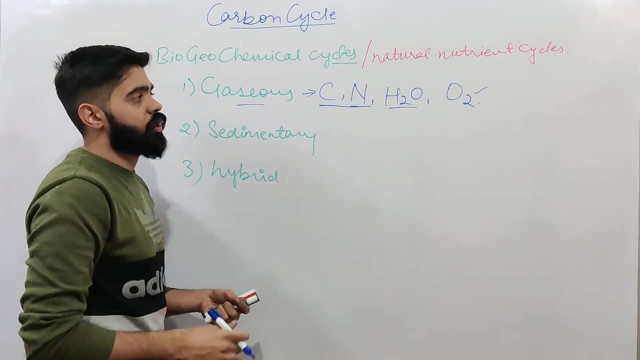 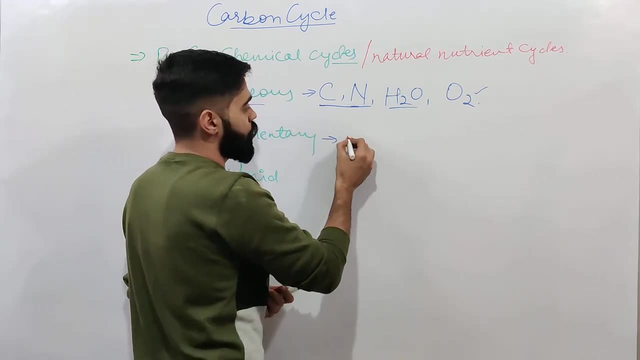 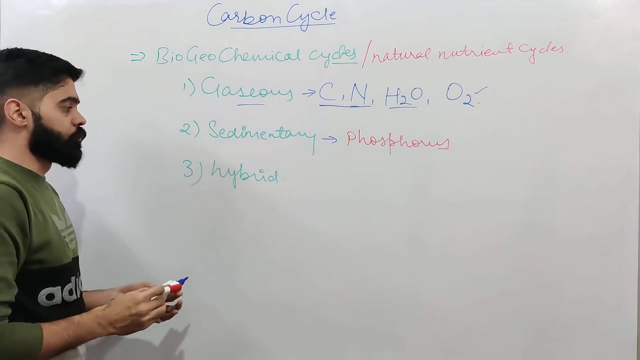 now we will study carbon in this. we have studied nitrogen cycle in class 11th. we don't study these two in this condition in sedimentary cycle in your class 2 ecology there is only one, and that is phosphorus. here is this phosphorus cycle. in hybrid conditions you have sulphur, so it can be sedimentary, it can also be gaseous cycle. it can be sedimentary, it can also be gaseous cycle, but the major proportion of sulphur which is uptaken by a plant is from the environment, from air. 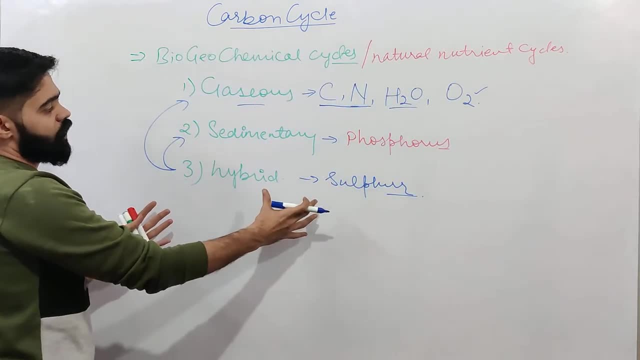 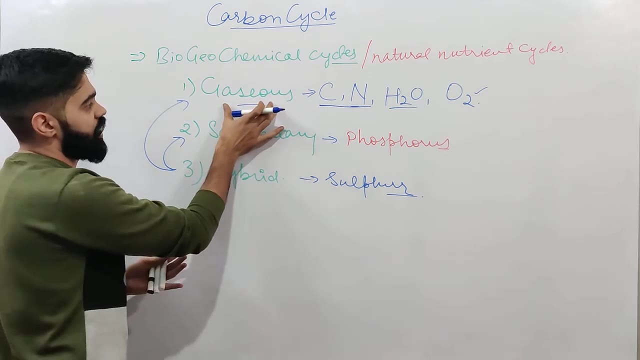 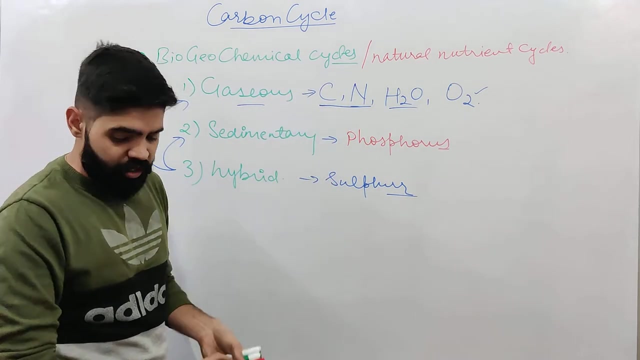 so it is present in environment in both of these ie, it is present in sedimentary lithosphere and gaseous in atmosphere, but plant uptakes more in gaseous form. is it clear? ok, so we are going to study about these. 3. 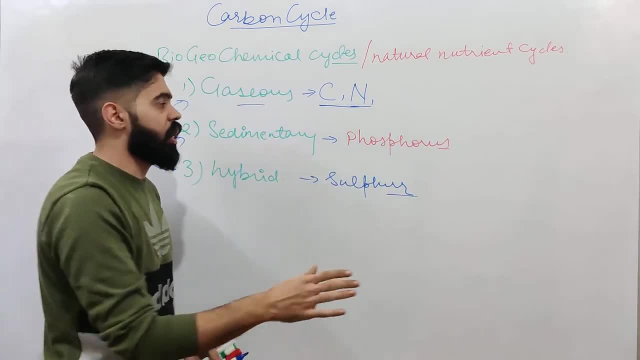 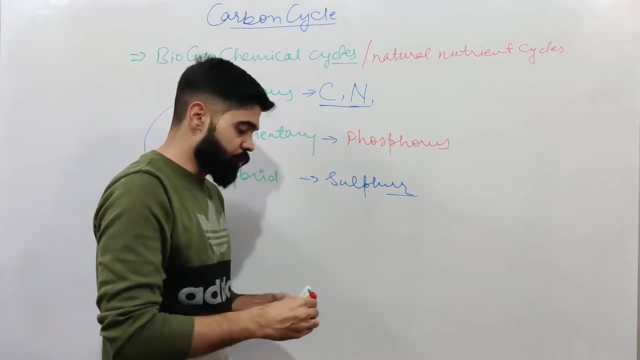 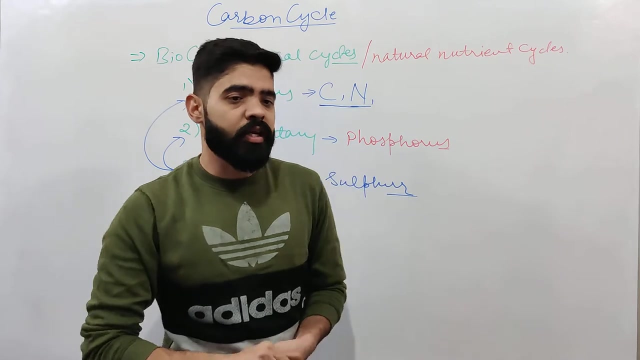 questions from sulphur cycle is never asked. questions from phosphorus cycle, carbon cycle and nitrogen cycle is often asked and from this also the mineral nutrition you did in class 11th nitrogen cycle was in very much detail which you can check out from class 11 mineral nutrition playlist. 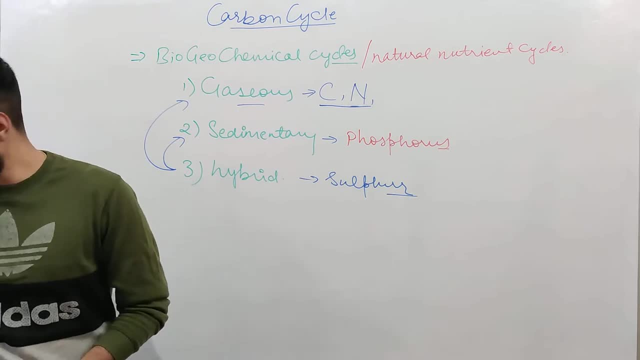 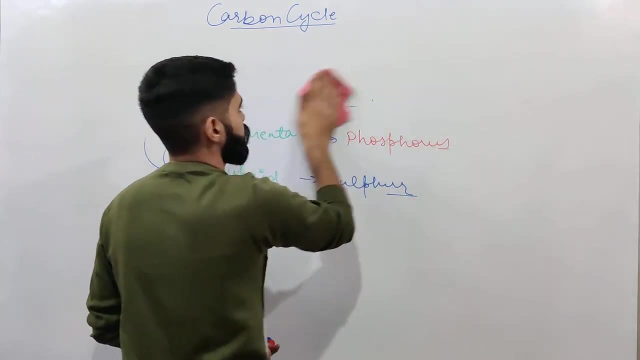 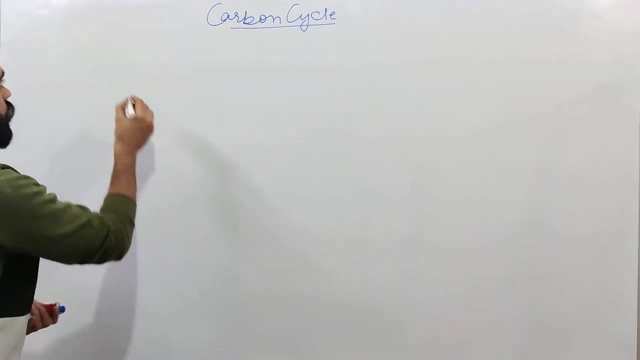 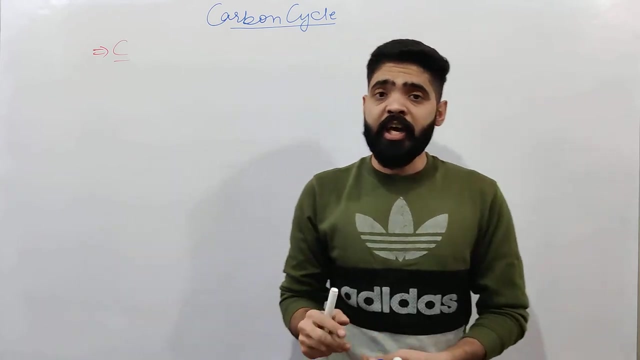 and we will start. for now. we are going to start with the carbon cycle. so the carbon cycle is first of all carbon, why it is used. carbon is the main backbone of every chemical, every chemical: amino acidcarbohydratefatsproteins. 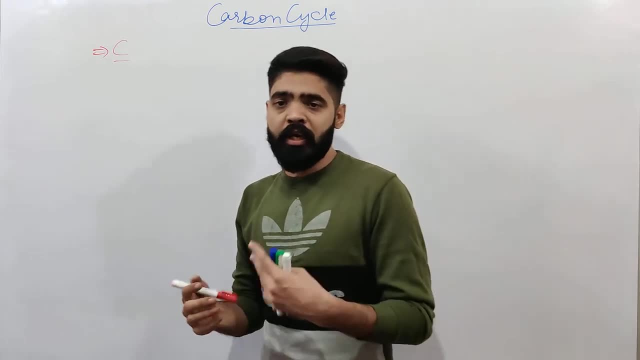 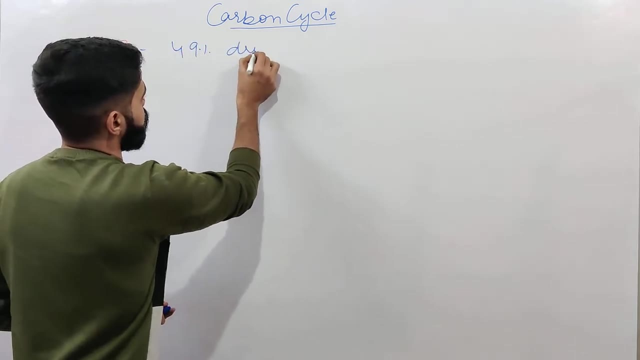 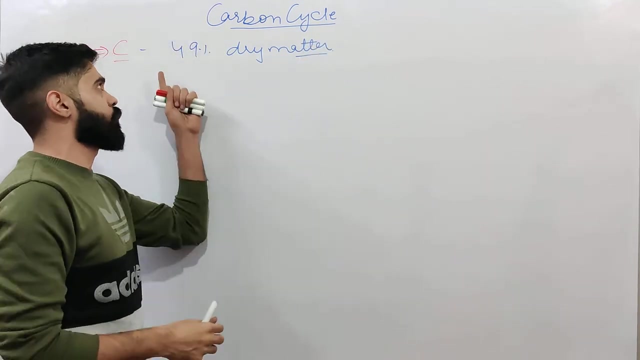 then we have vitamins, whatever you take name of. so in all things, carbon is present as a backbone and there is 49% of dry mass. 49% of dry matter of any organism is made up from the carbon. what is dry matter? why it is calculated. 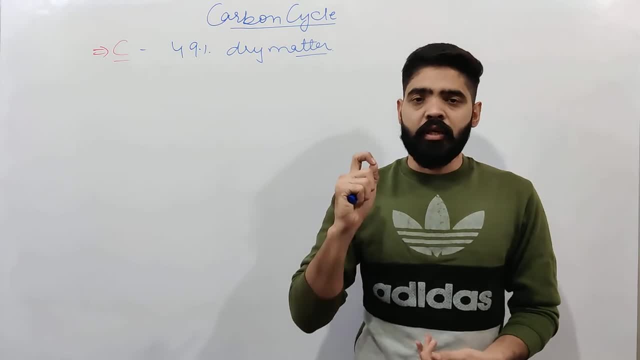 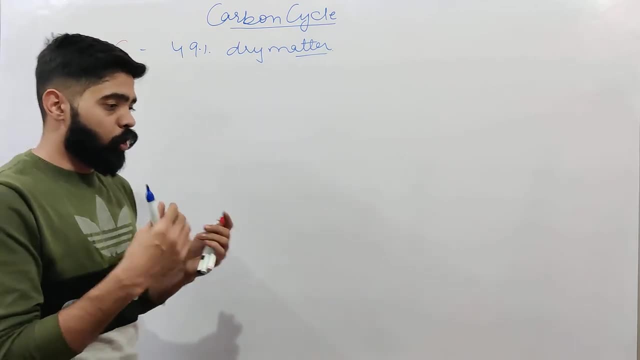 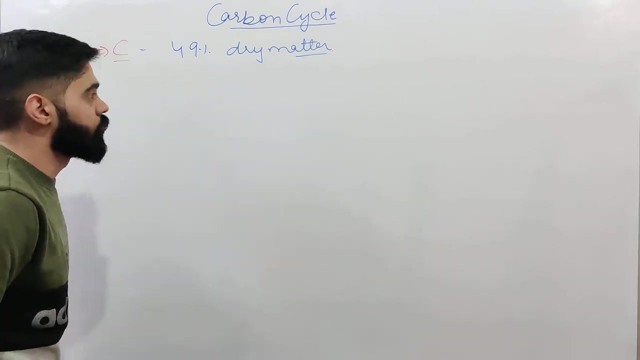 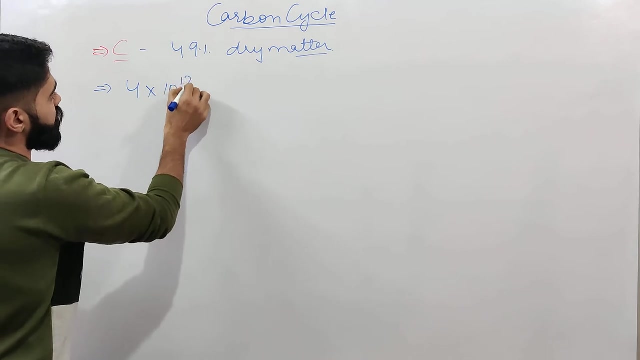 because it is best suitable biomass unit taking as dry matter because of removal of water, because of removal of molecular water which is present, or the water which is present inside if moved out. so that is dry matter. apart from this, 4 into 10 raise to power 13 kg. 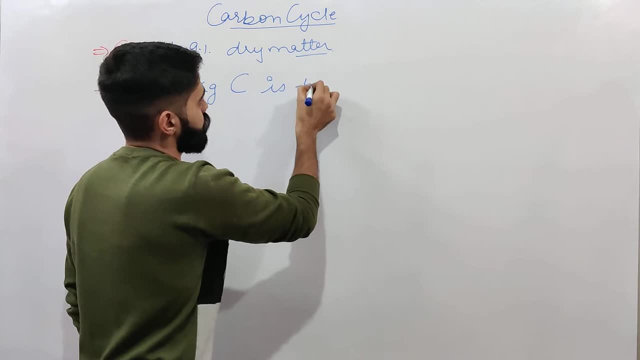 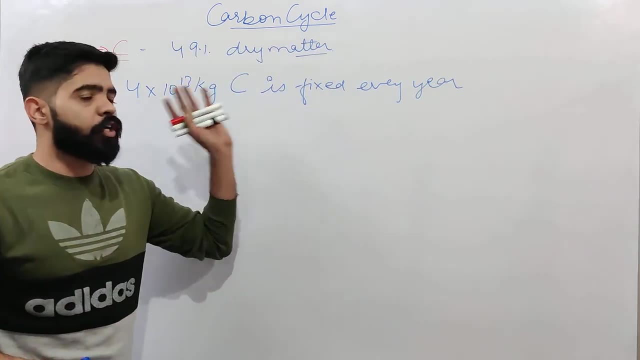 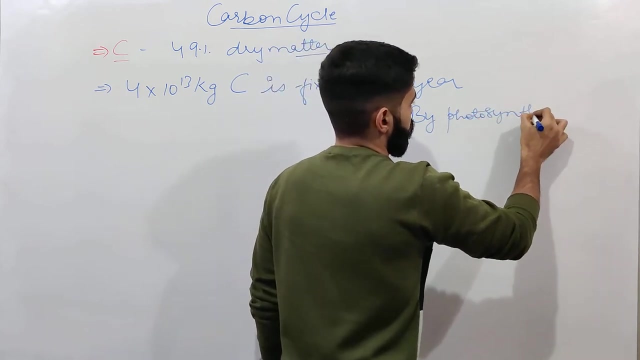 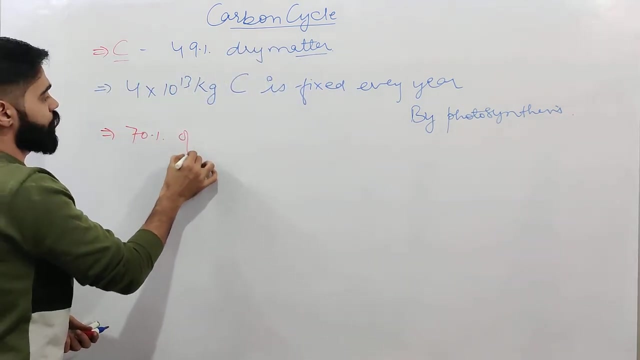 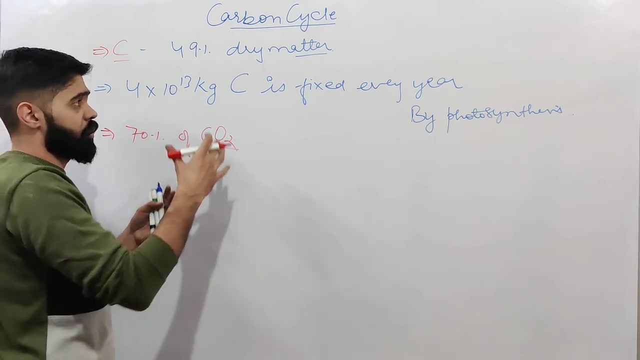 carbon is fixed every year, is fixed every year by photosynthesis, and 70% of this carbon- or you can say CO2, because which is the main carbon source present in any environment, in our environment, any environment- we do not give a damn about any environment- carbon dioxide is main carbon source. 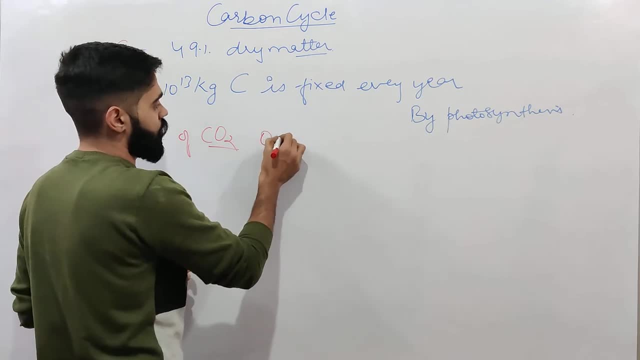 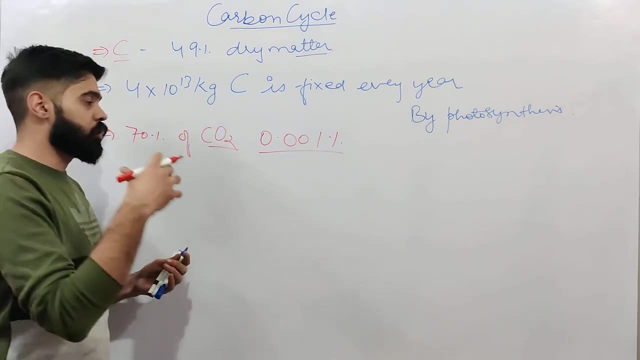 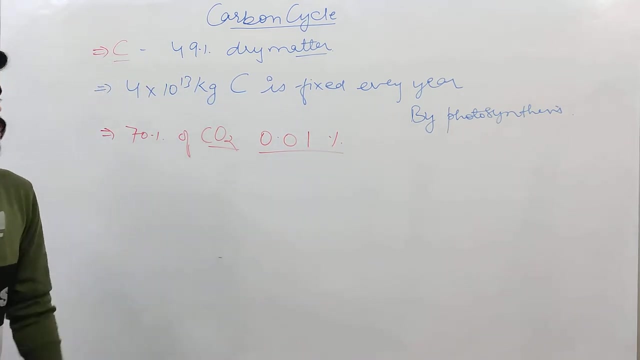 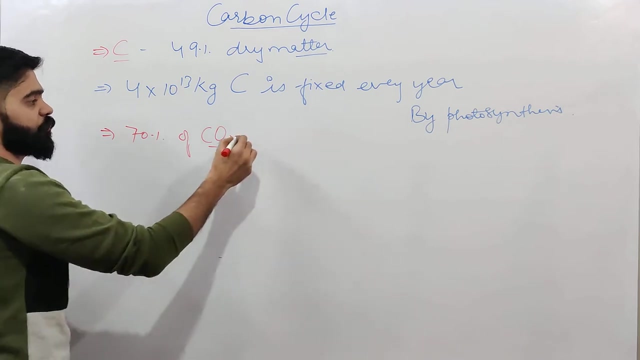 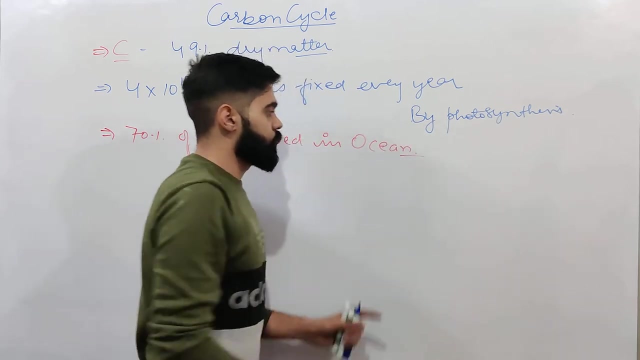 in atmosphere present and its concentration is particularly 0.001%. where is this in the environment? let me tell you: 0.01% clear this. but still, 70% of this carbon dioxide is fixed in ocean. now, this was a question in NEET. 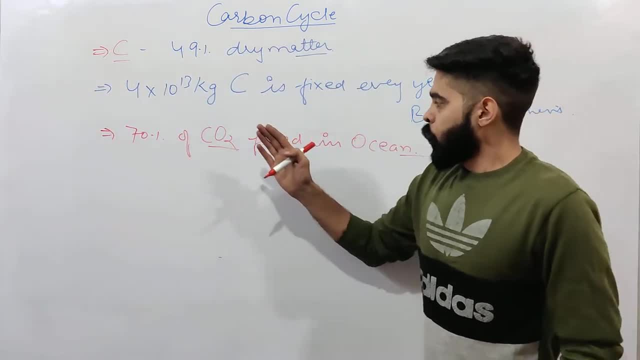 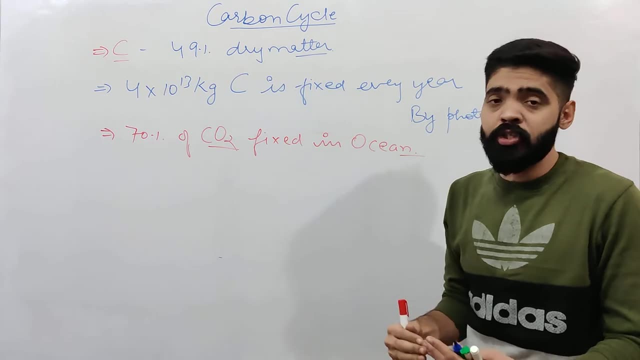 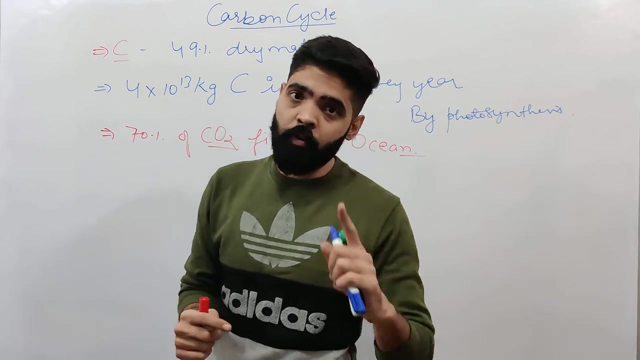 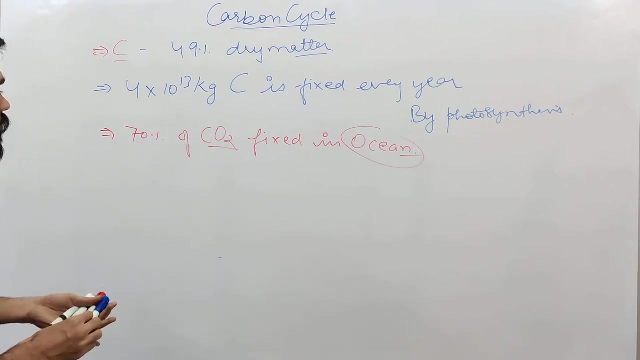 2005 or 2007, I think. carbon dioxide: 70% of amount of carbon dioxide or carbon is fixed in below were given 4 options: lithosphere, atmosphere by photosynthesis in ocean, so correct answer will be in ocean here with this. after this, we have: 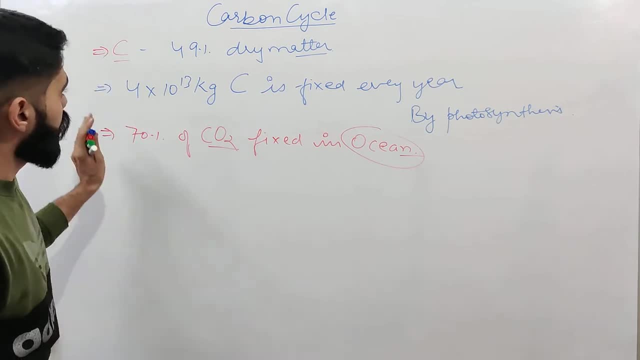 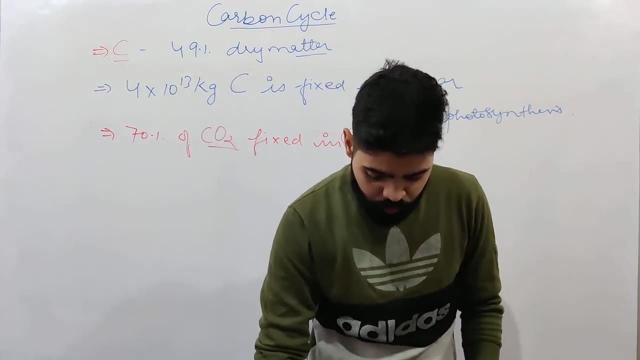 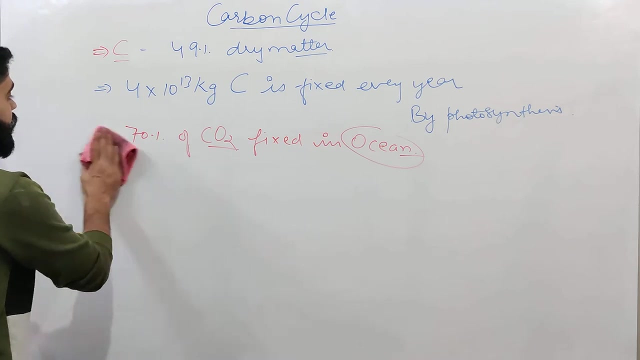 now, this was the fixation part and every single thing which is present in your NCRT. let me check NCRT. this is completed. so after this, directly we have carbon cycle. it is a gaseous type of cycle and the main source of input. see every cycle. 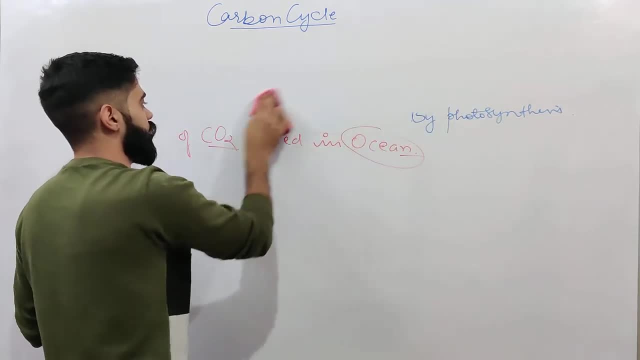 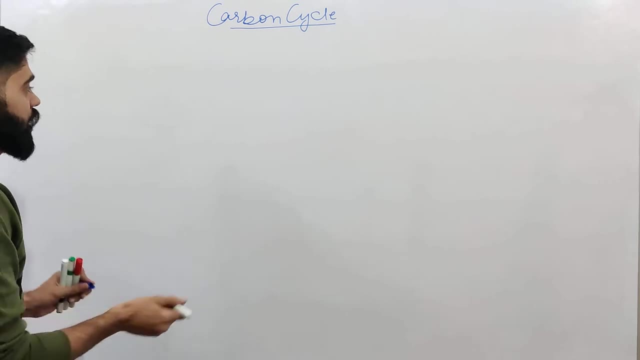 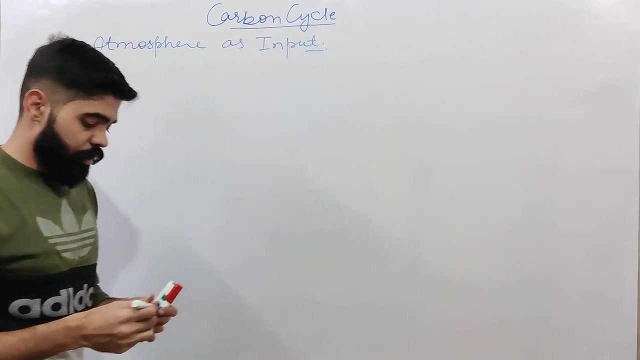 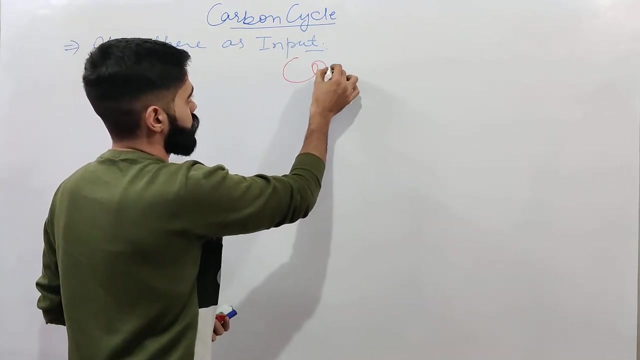 which is present in environment have certain input and output. yeah, input and output. so, input in any biogeochemical cycle in case of carbon cycle, is atmosphere. clear with this. in case of carbon cycle, atmosphere is input and it is having carbon dioxide present in environment. clear with this. 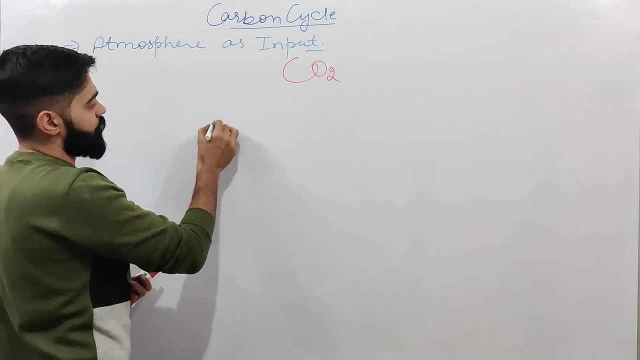 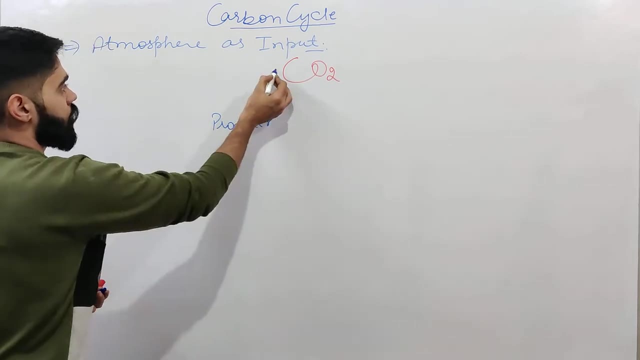 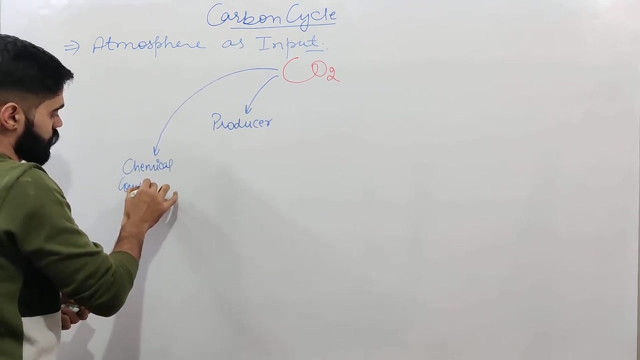 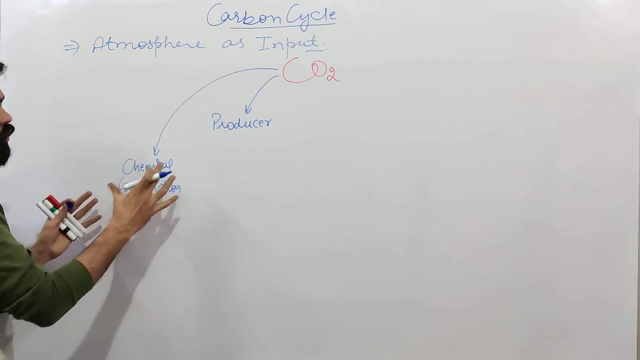 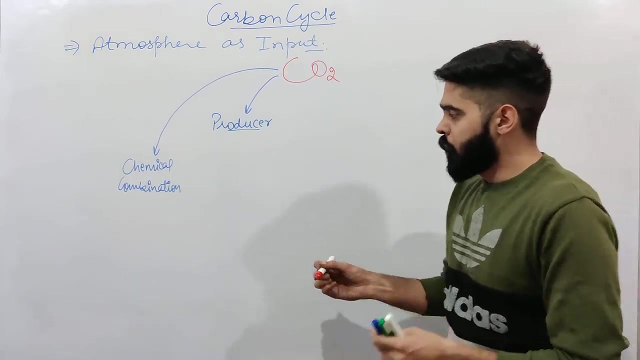 now, carbon dioxide is uptaken by producer, so it is uptaken by producer, or there can be chemical combination, chemical combination. so these two things are for the fixation of carbon. now carbon is fixed by producer and chemical combustion is also fixed by which chemical combustion is made from there. 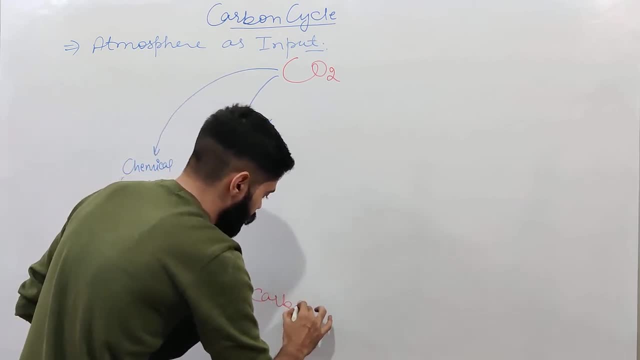 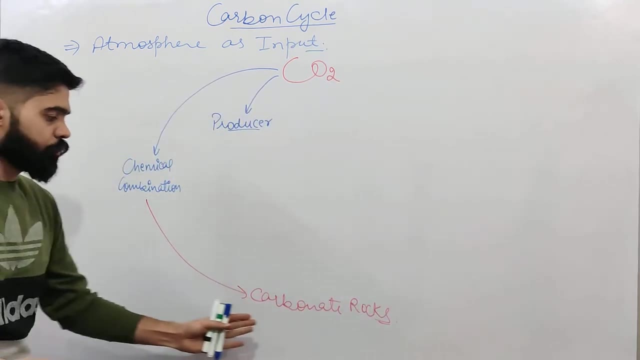 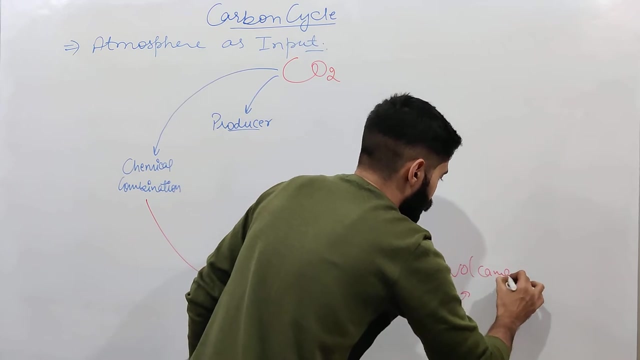 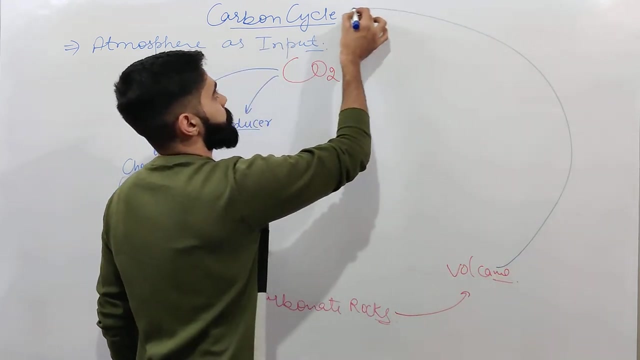 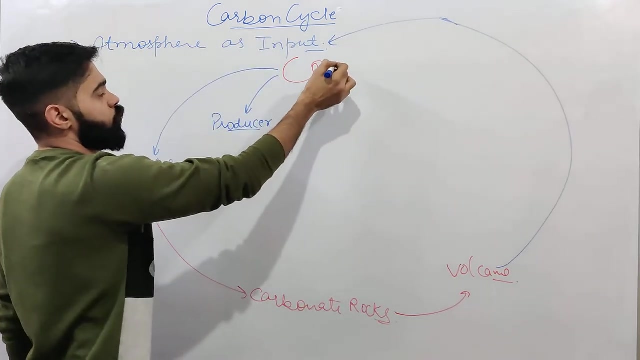 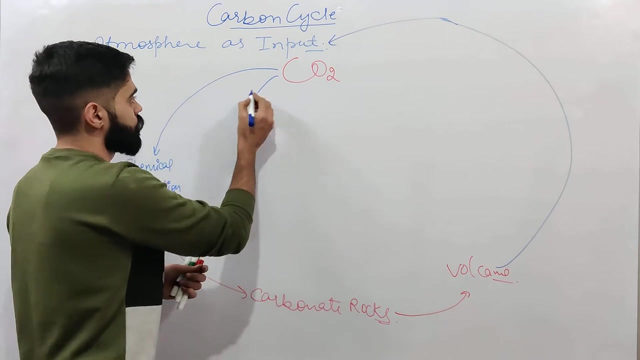 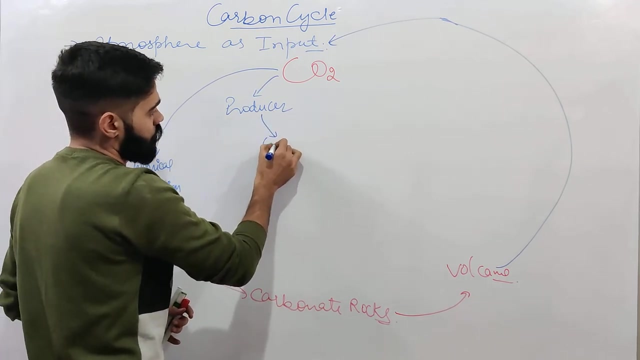 carbonate rocks. clear with this. this chemical combination forms carbonate rocks and these carbonate rocks are present in a volcano. so whenever any volcanic eruption happens, the carbon is moved out into the carbon dioxide of environment. clear with this. now, this producer. what can happen with producer? this producer can be eaten by consumer. 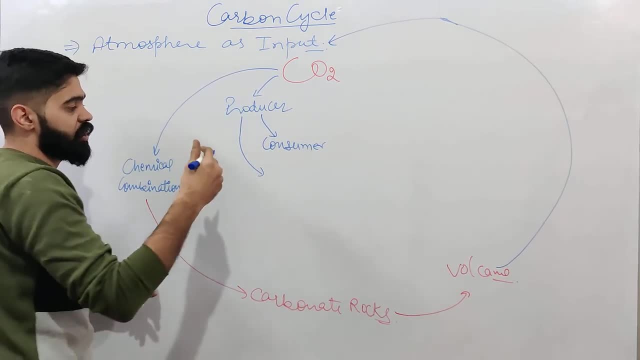 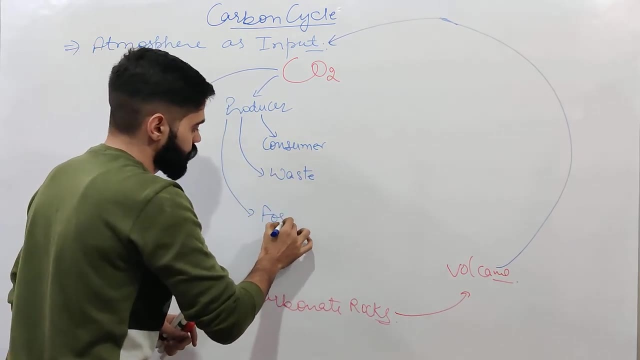 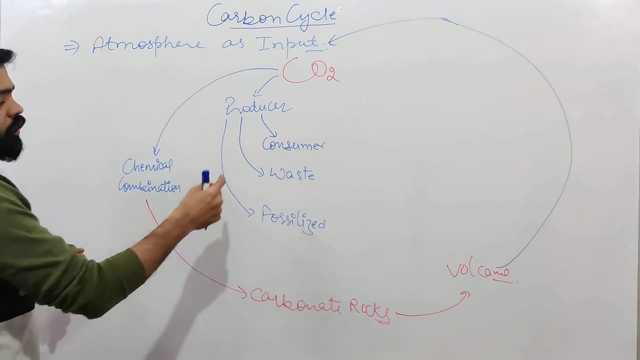 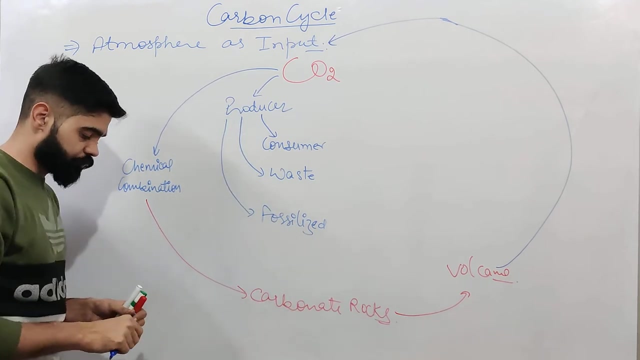 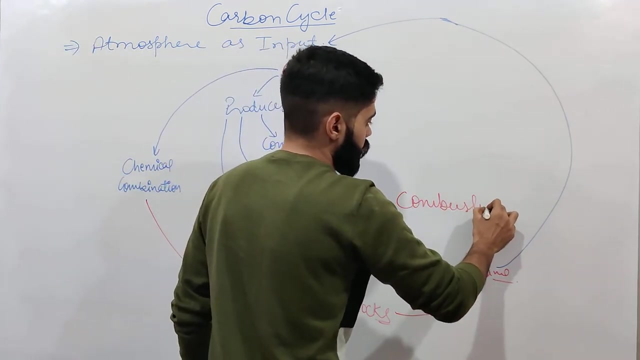 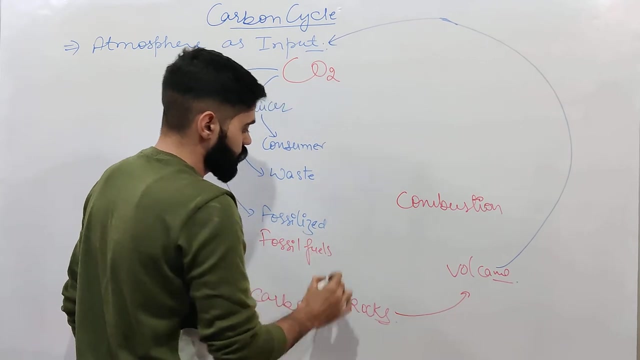 one thing. second, this consumer can die and waste can be produced. this consumer can be fossilized. these three things clear with this. this consumer, one waste material, two, that is litre, or this producer can be fossilized. now, fossilization always undergo combustion. this is called fossil fuels. 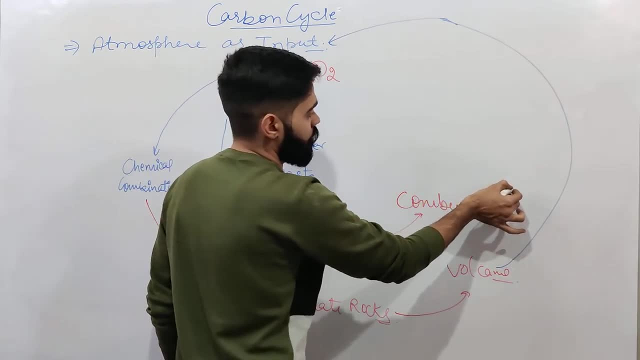 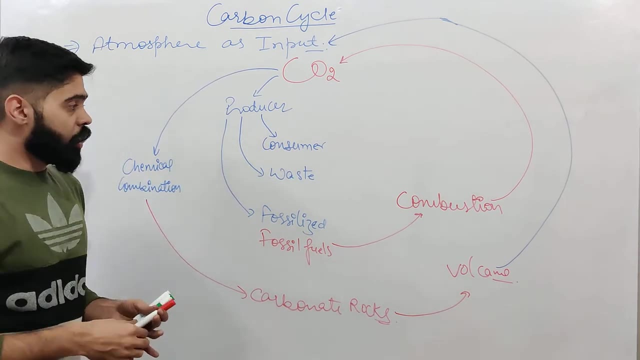 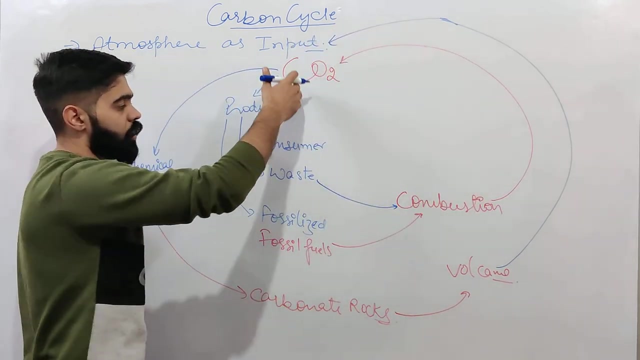 this fossil fuel combustion, and combustion will always gives out, gives out CO2 clear. with this, ok, now we have the waste material which can also undergo combustion, again going into as carbon dioxide in environment. these consumers can also be fossilized waste material. now producer can be a waste material. 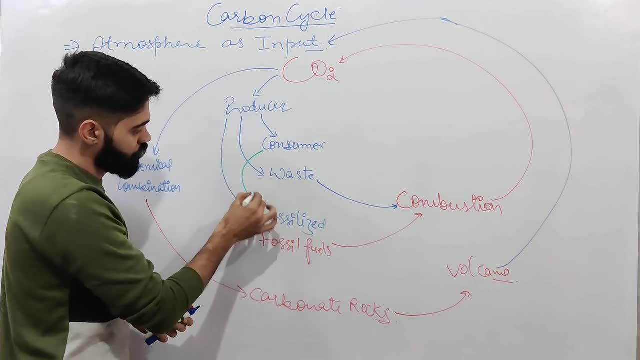 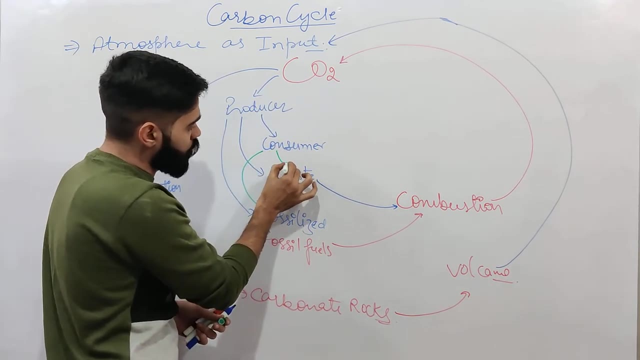 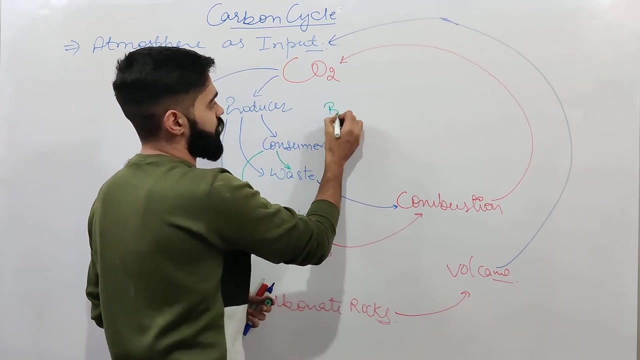 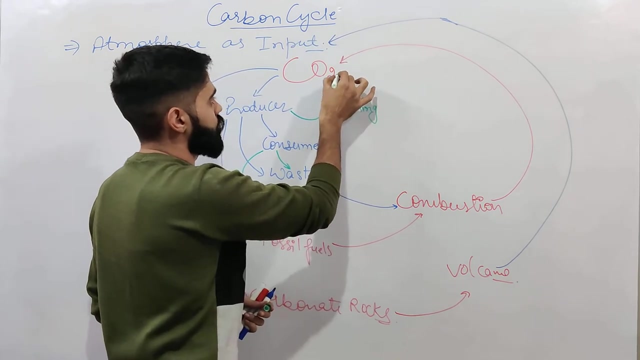 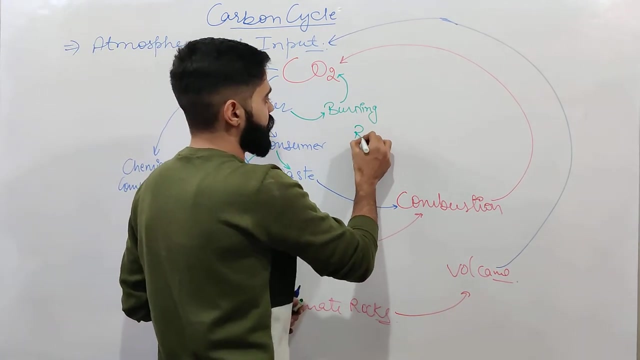 but consumer can also be a waste material. now, producer can be a waste material, but consumer can also be a waste material. so now we have a a, a, a, a, first a, a, a y, an, a, a, a, a, c, a, s, a a r a a e. 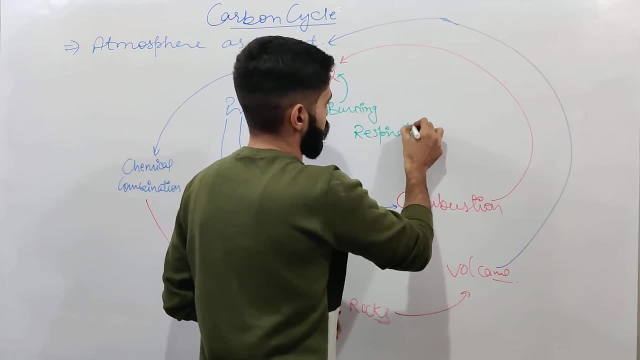 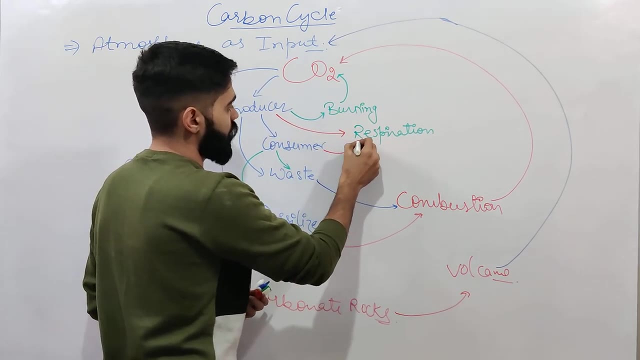 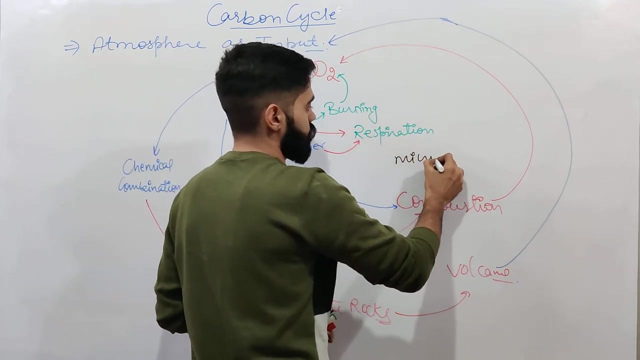 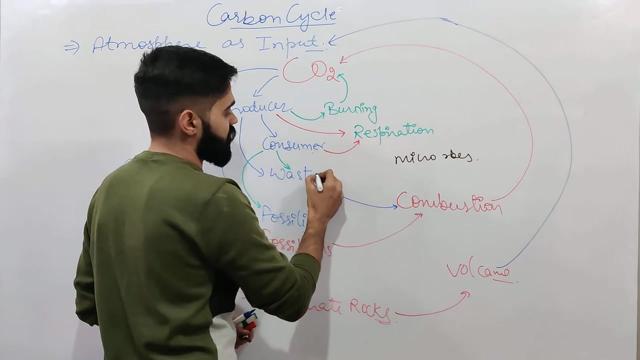 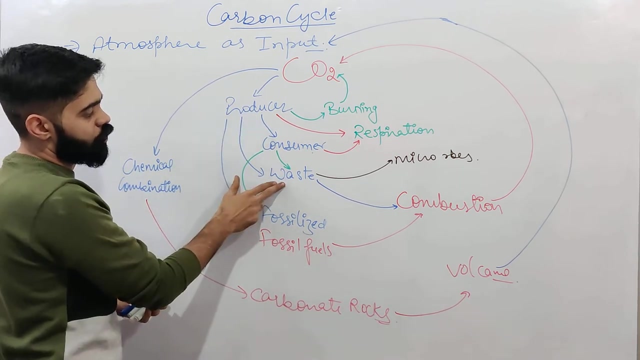 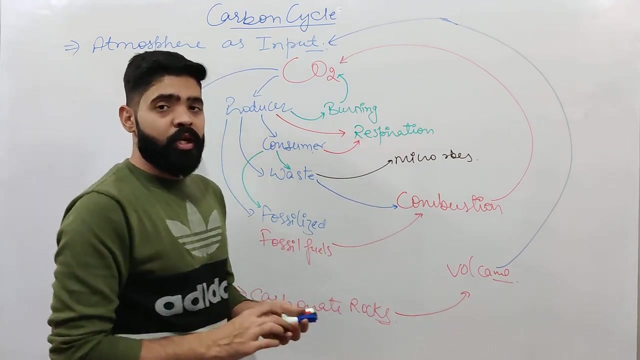 b, a, a, a, a, a, s, a, c, a, r, a respire. and there is one more thing that is added into this is microorganism microbes. so consumer after death can go to micro microbes. producer after death or waste can undergo to decomposition by microbes and aerobic respiration will. 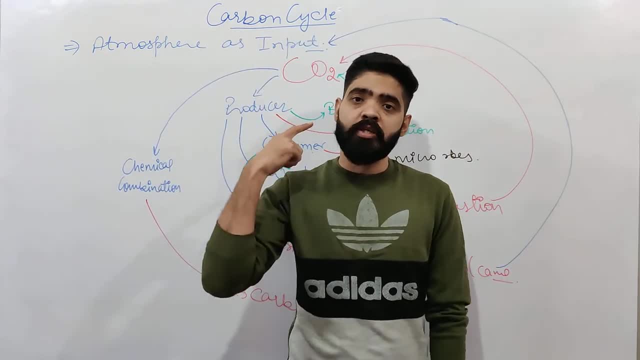 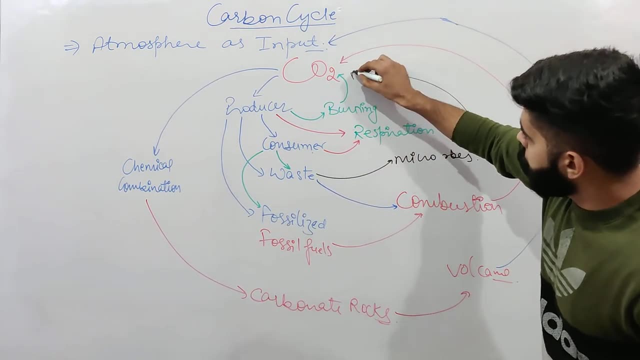 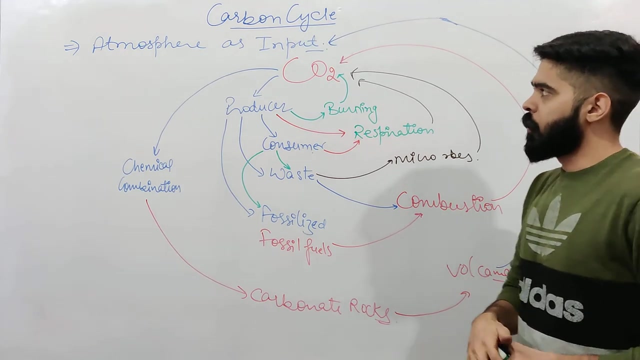 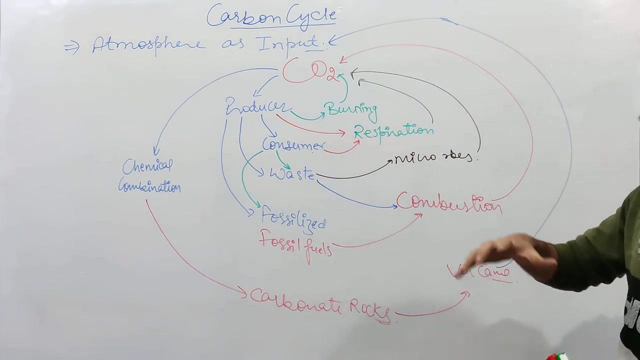 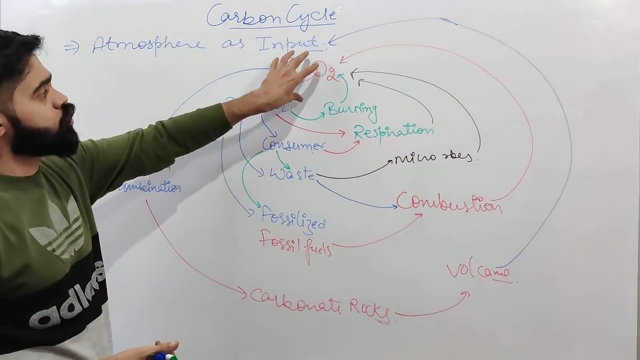 always lead to formation of two things: water, molecular water and carbon dioxide. so there are two ways of fixing carbon dioxide which is present in the environment. one is chemical company combination, second is producer and there are five different ways of output. what is this? there is one source of input, that is, environment, and there are 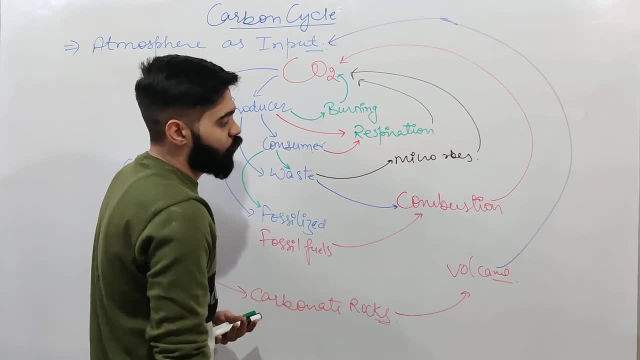 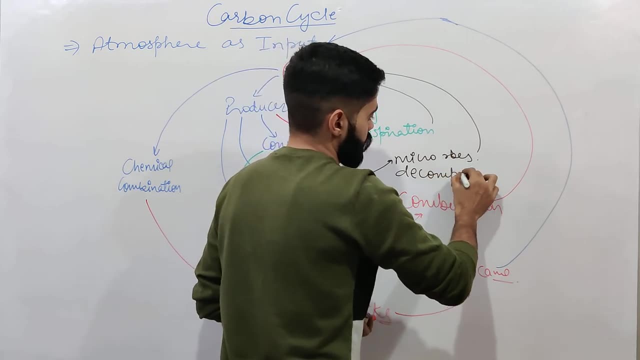 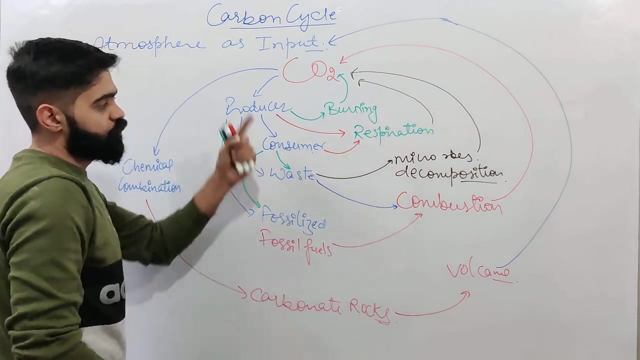 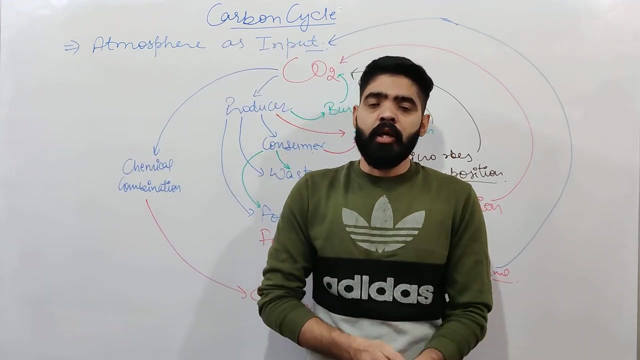 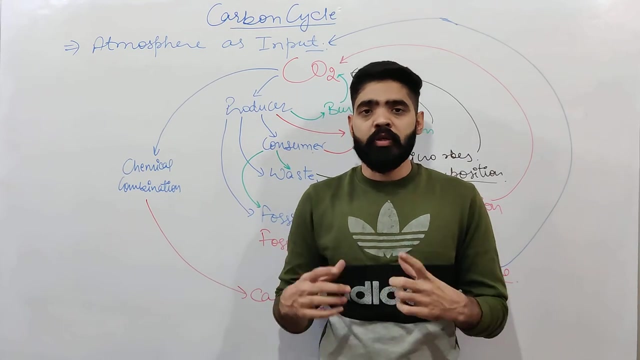 five different sources of output: volcano, volcanic eruptions, combustion, microorganism, decomposition like down respiration and burning. these five are output sources. so thank you so much, everyone for today. tomorrow we will be studying about this phosphorus cycle and ecological and environmental services that we are taking, and a small estimate of. 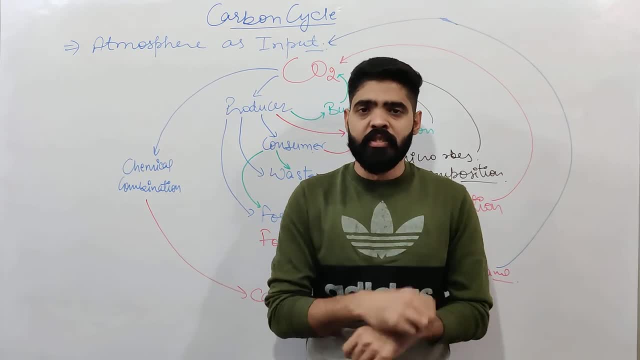 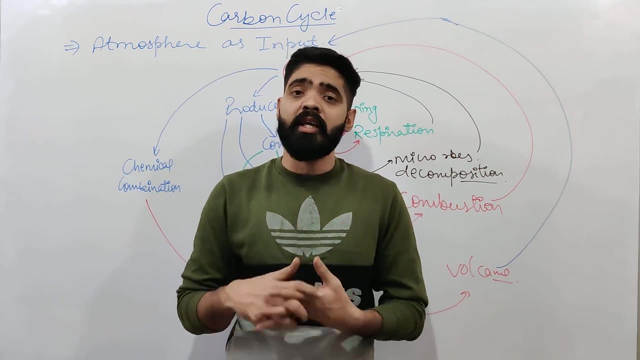 the studies that we are taking. If you remember, you will get questions from that too. Whatever is given in your NCRT, whether that data is old or how it is, if the NCRT is not updated then it is not the student's fault, but still, they are giving the questions based. 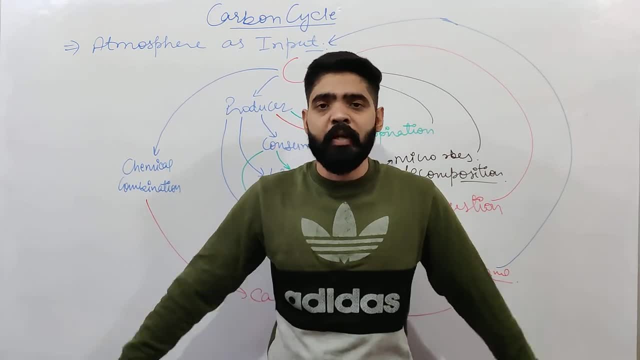 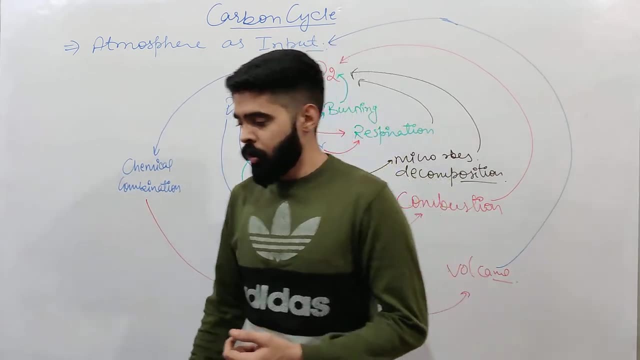 on the data that is provided in the ecology. To remember, in these chapters you have only data, plus some very simple processes that you also learn from small classes. Thank you so much. everyone, Make sure to give a thumbs up.